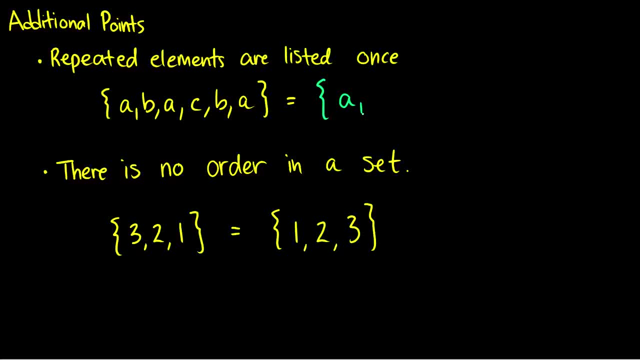 is repeated three times. we only write it once. B is repeated twice, we only write it once. and C is repeated once. So this set A, B, A, C. B A is the same set as A B C and they would both be. 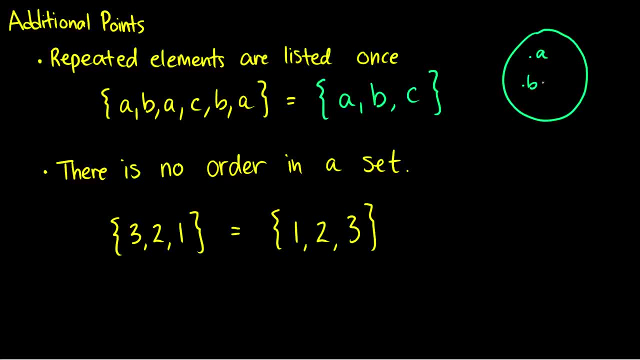 drawn as circles with some element A, some element B and some element C. In other words, we don't care about the set A, B, A, C, B, A, and they would both be drawn as circles with some element A. 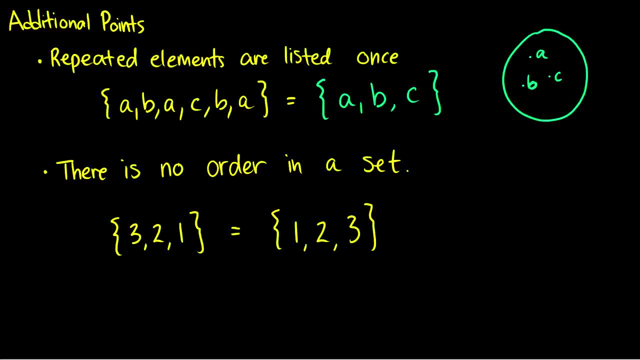 so we don't care about the amount of numbers of these things in there. We don't care if there's three A's, we don't care if there's two B's, we just want to know what's inside our circle. There's also no order in a set and in a diagram. this is easy to see because there's no order in. 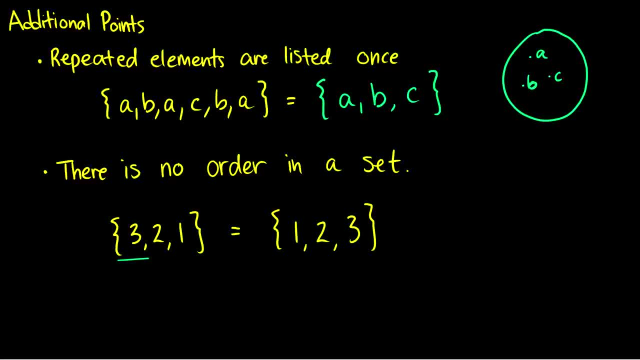 a circular diagram. but essentially, the set 3,, 2, 1 is the same thing as the set 1, 2,, 3, and that's also the same thing as the set 2, 1, 3,, so on and so forth. There's no order to these sets. 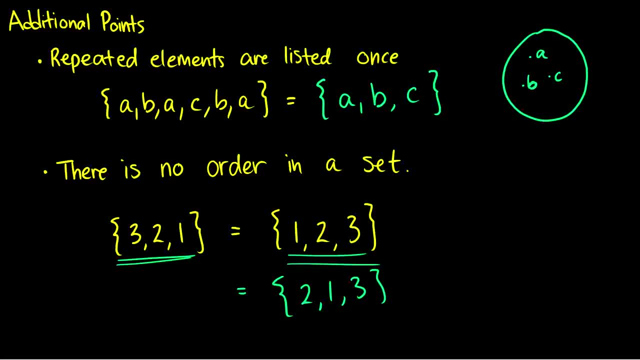 So those are two pretty important parts. Usually on an exam, you might be given a set that has repeated elements and they might ask you: how big is this set, How many things are in it? And if you're not sure about repeated elements then you might get the wrong answer. 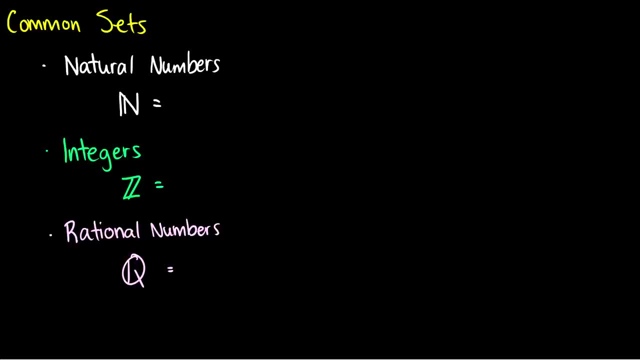 There's a few common sets that we should talk about. One of them is the natural numbers. The first time I made this video, it was controversy, and there's still some controversy, but there's two ways to do the natural numbers. One of them is to start with 0, do 1,, 2,, 3, all the way up forever and ever. 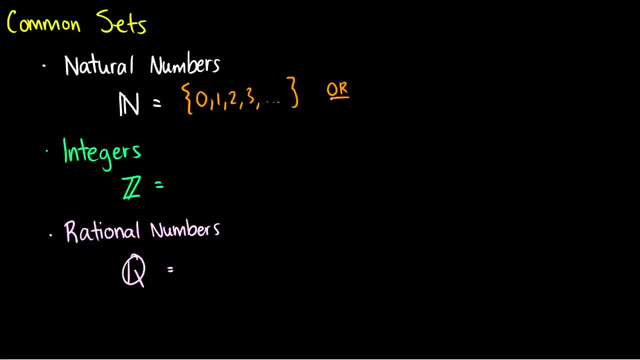 Another group of mathematicians starts the natural numbers with 1,, 2,, 3, so on and so forth. I'm going to refer to the natural numbers starting with 1 as the positive integers and when I talk about natural numbers anywhere else, 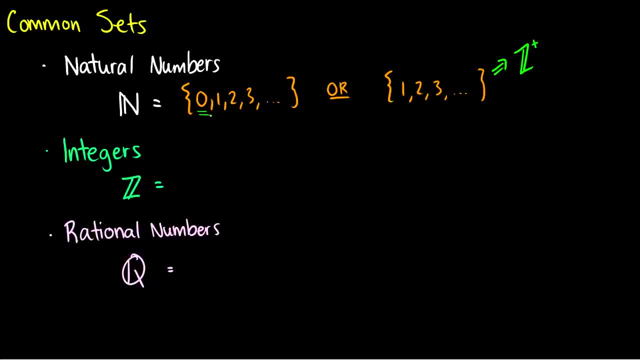 I will usually mean including 0, but I may be more specific about it. So I will specify whether it includes 0 or not, but typically with 1,, 2, 3, so on and so forth. I'll use z plus. 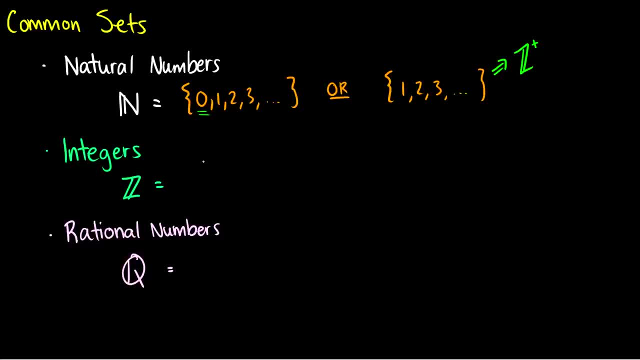 The integers are a set of numbers which are either positive or negative and they're whole numbers. so all the way from negative infinity- negative 2, negative 1, 0, 1, 2, all the way to positive infinity. so that is z. 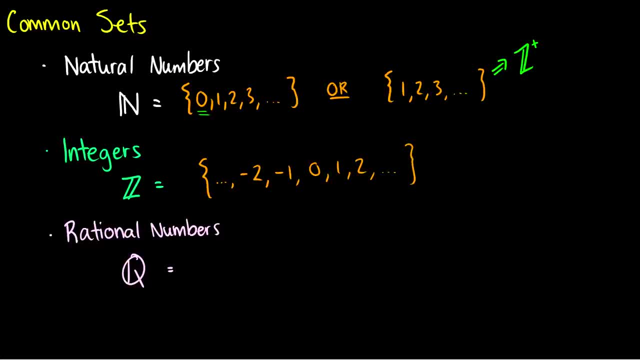 That's a very important notion which we use a lot in discrete math And then rational numbers. Oh, these are kind of hard to list, so I'm going to cheat a little bit for now and I'm going to say: well, we have like 1 over 1, 1 over 2, 1 over 3, 2 over 3, so on and so forth, and in a few slides we'll figure out a better way to write this. 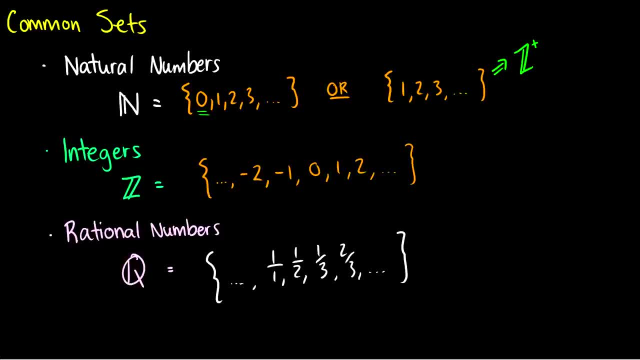 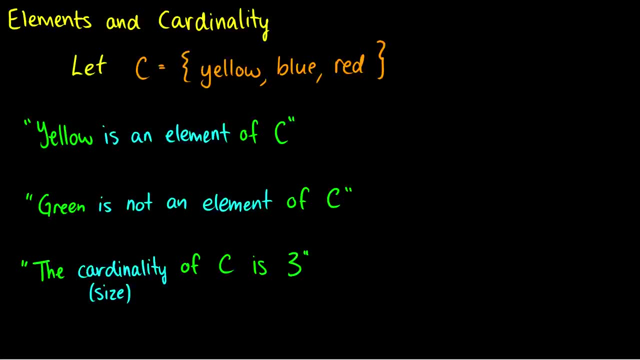 So of course, rational numbers are any numbers you can write as a fraction. So elements and cardinality. Now we know what sets are. Now we know some additional pointers about sets. We know some common sets, But we want to be able to talk about the things in those sets and how big those sets are. 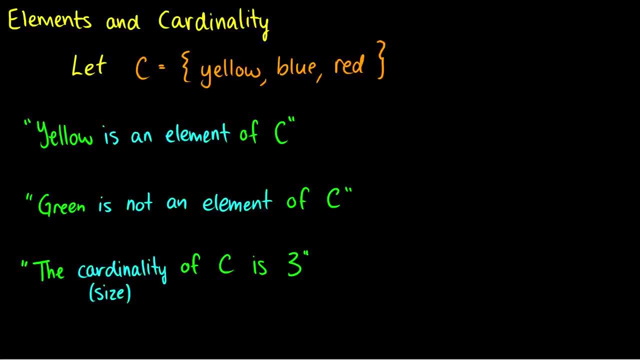 So I have C and I have a set containing yellow, blue and red. So these are the primary colors. In fact, sets don't have to be all mathematics. They can be words too and have meaning in the real world. 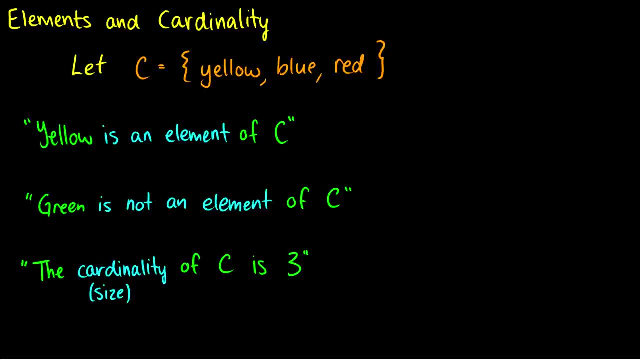 So I want to say something like: Yellow is an element of C And this means that yellow is inside of our set C. Now how do we write this? Well, we have an element, yellow, and we want to say it's part of a set C. 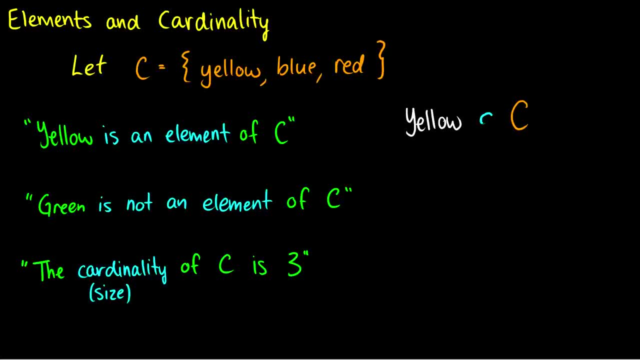 So in order to write this in notation, we use this epsilon. So yellow is in the set C. What about saying green is not in the set C? So I want to say green is not in here. In fact, we don't see it in the set C. 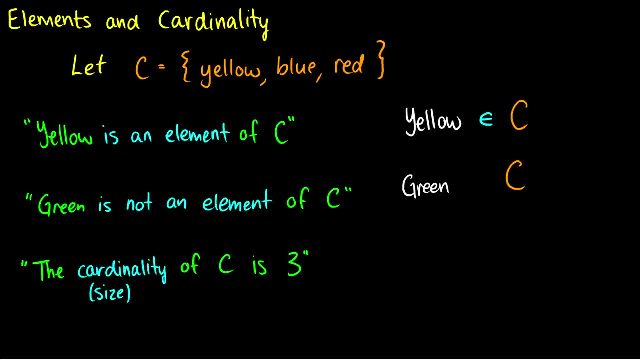 So what do we do to say green is not in C? Well, we use the set membership symbol and we just put a line through it To mean green is not in our set C. How do we talk about the size of this? 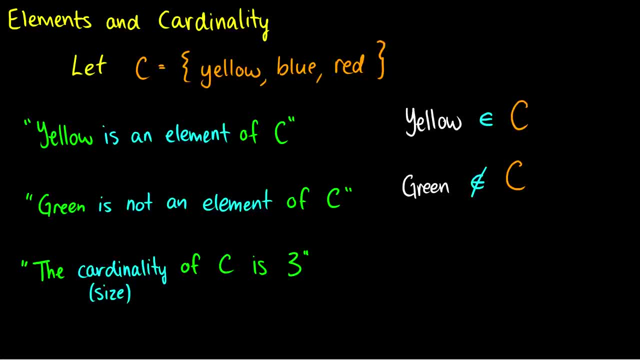 How do we say the size of C is three, Which means the amount of things in C is three. There are three different elements in C. Well, we just draw these absolute value bars around it. So we say that the absolute value or the size. 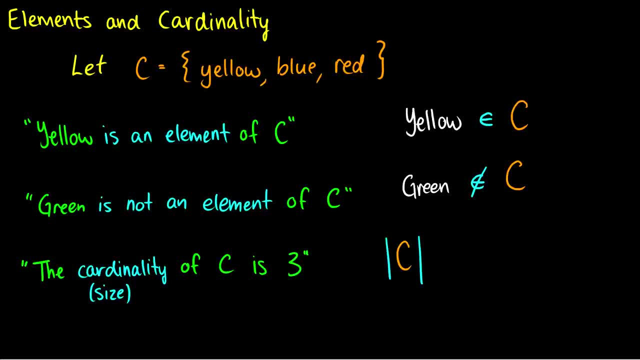 of C is equal to three, And that says that the cardinality of C is three. So now we can talk about whether things are inner sets and how many things are inner sets. Now there's one particularly interesting set that contains nothing in it. 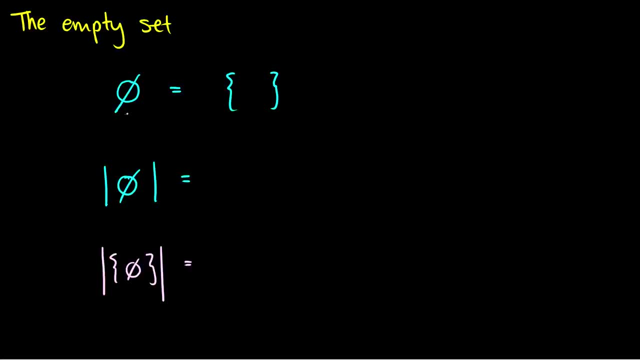 This is called the empty set and this is written with this symbol, And if I wanted to write it in the set notation with curly braces, it would look like this: It has a left curly brace, a right curly brace and then there's nothing inside of it because it's empty. 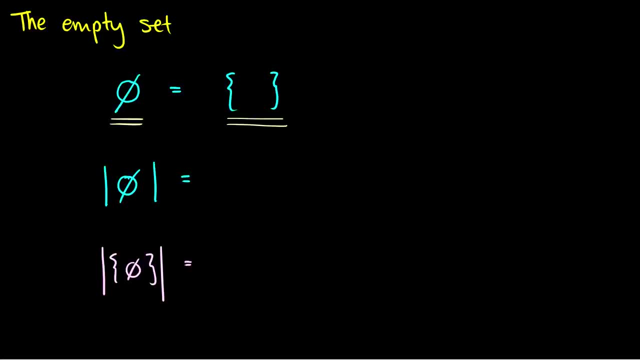 So what's the size of this set? Well, there's nothing in it, So the size of it is zero. And there's only one set that has a size of zero, and that is the empty set. So here's a question. 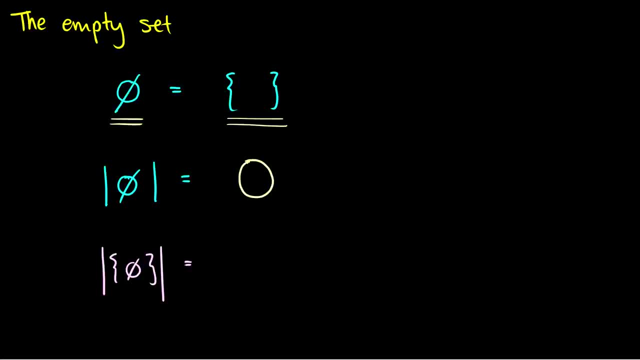 And I'm throwing this right at you right away, because this trips people up all the time- What is the size of the set containing the empty set? So I'm asking: if I have a set containing the empty set, what's the size of that set? 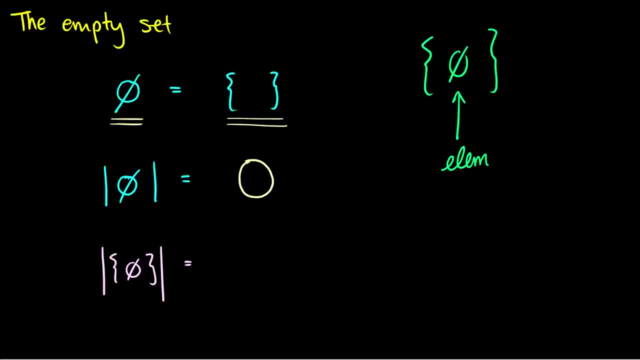 Well, this empty set is an element of the larger set, So the size of the set containing the empty set is one, because this set itself, this big set, has one element: It has an empty set as an element. So sets can have sets as elements. 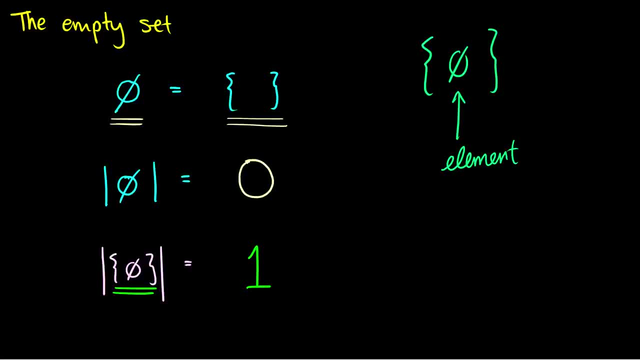 We'll see another example later, But typically I like to look where the commas are. So if there's like a big set, then a comma, then another big set and that's all that's in the set, then there'd be two elements. 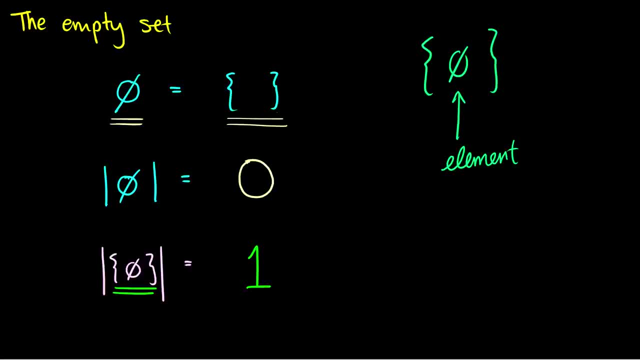 In this case, we have these empty braces, but there's something inside of it, So therefore there's an element in that set. This is different, of course, than the size of the set containing nothing. This would be zero. So we can see the contrast between these two sets. 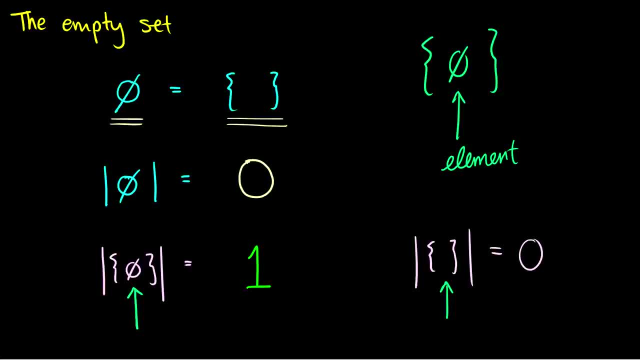 This is the empty set on the right, while this is a set containing the empty set on the left. The left one has a size of one, the right one has a size of zero, and we can see the differences visually. Okay, so that's the empty set. 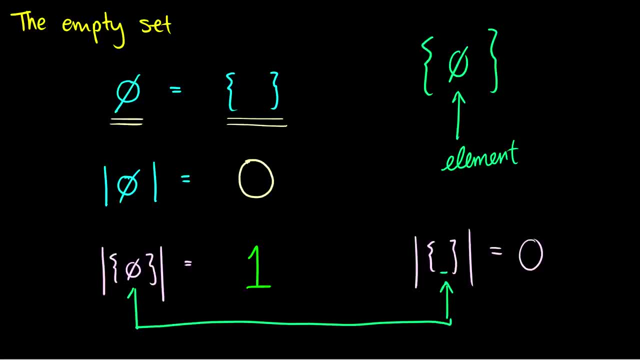 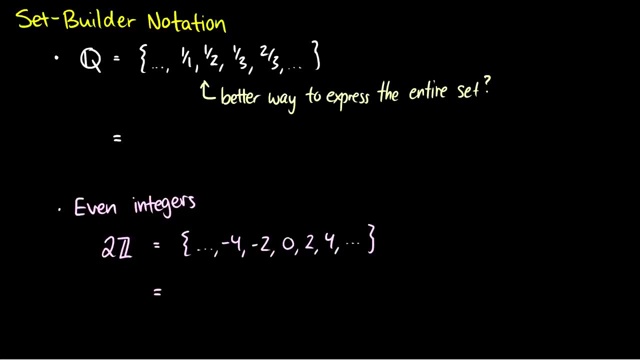 There'll be more questions about the empty set when we get to the subset video, so more tricky stuff will happen there. The next thing we should talk about is set builder notation. So before I introduce the rational numbers and I said, oh, it's one over one, one over two. 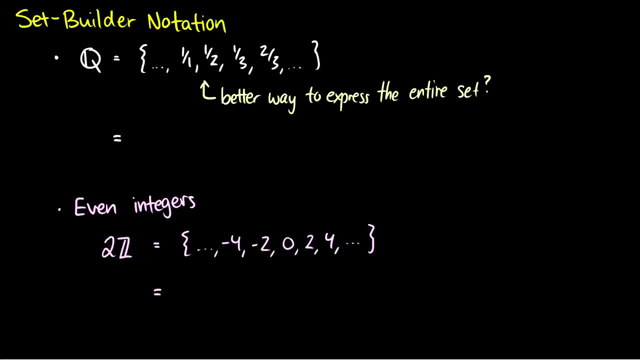 one over three, two over three, so on and so forth. there's got to be a better way of representing this entire set, And this is set builder notation, or we can call it maybe predicate notation, where we define elements as variables. 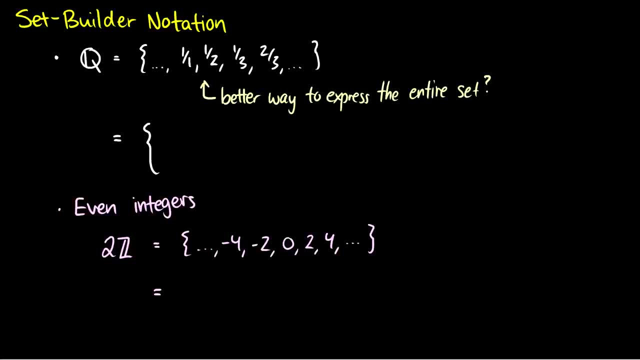 So, for instance, I can say: this is the set containing elements that are of the form m over n, such that. so this straight bar means such that. and now I'm going to give a rule. So the left is like the form that it takes. 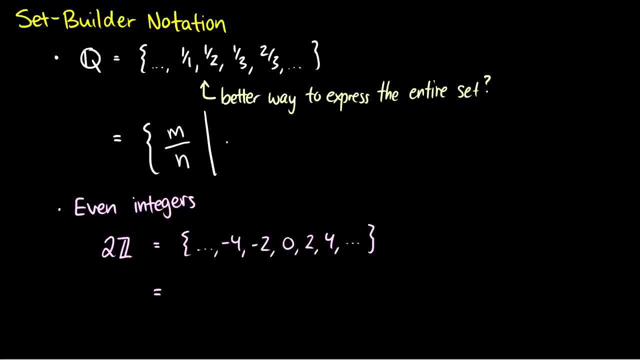 and on the right side we're going to give it a rule. We're going to say that m and n have to be integers and also n has to not be zero, so that way we're not dividing by zero, And this expresses the entire set of rational numbers. 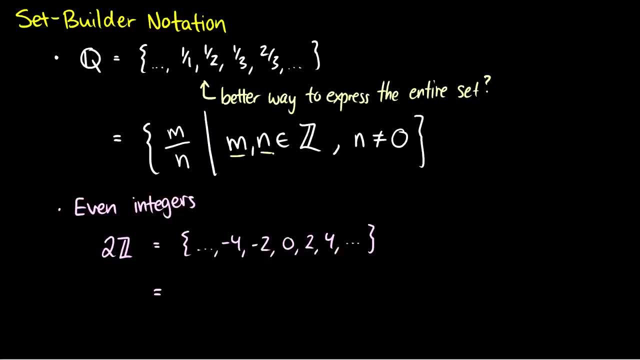 I'm saying: look, take any two integers, m and n. we can put m on top of n and as long as n isn't zero, it's going to be in that set. So I'll do another example with even integers. 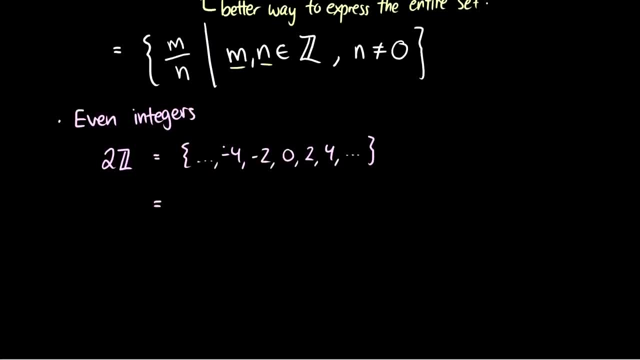 So we can write all the way to negative infinity, negative four, negative two, zero, two and four, so on and so forth to infinity. or we could do this in set builder notation So we could say: this is the set of. 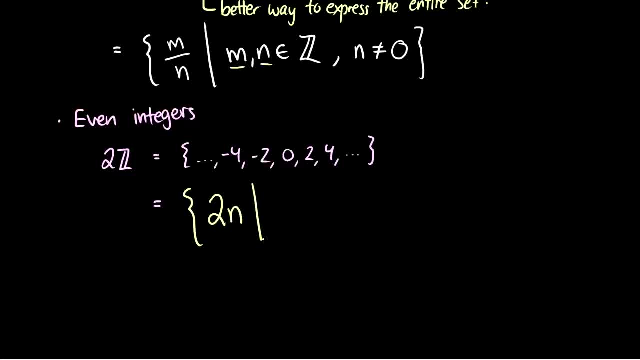 let's put two n, such that n is an integer. So what this means is we take an integer n, so let's say we take one, then in our set we add two times that integer, so two times one, so we add two. 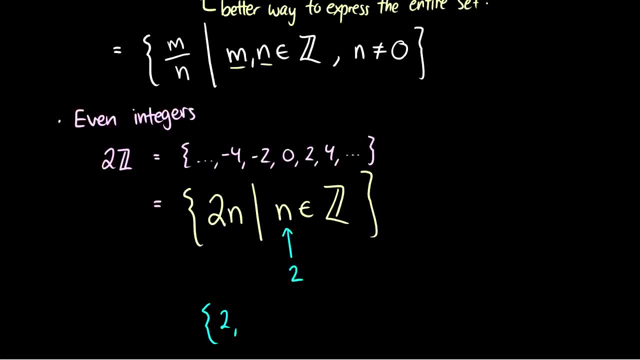 Let's say we take two, then we take two times two and put in our set four. Let's say we take negative one, then we take negative one times two. we add negative two in our set as well, And this just goes on forever. 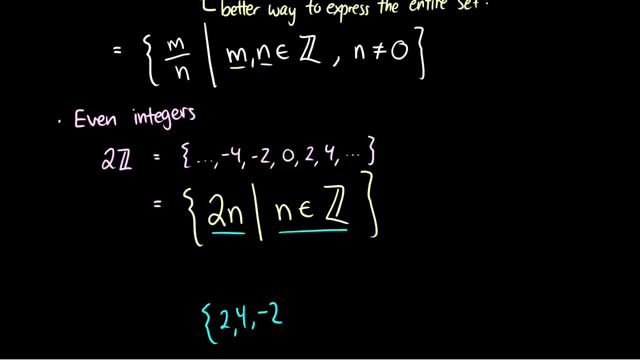 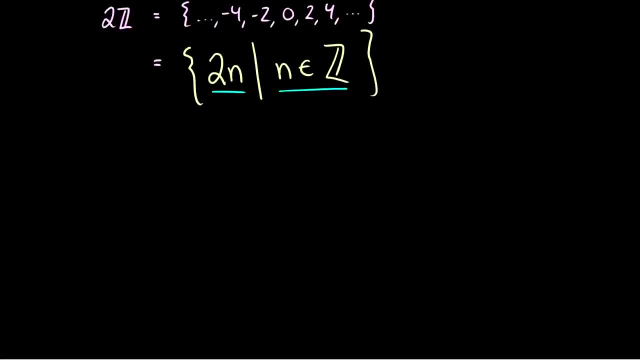 So for every n that is an integer, we add two n to our set And that gives us the set of even integers. So here's a more linguistic example, so something we can apply in the real world to see how this notation works. 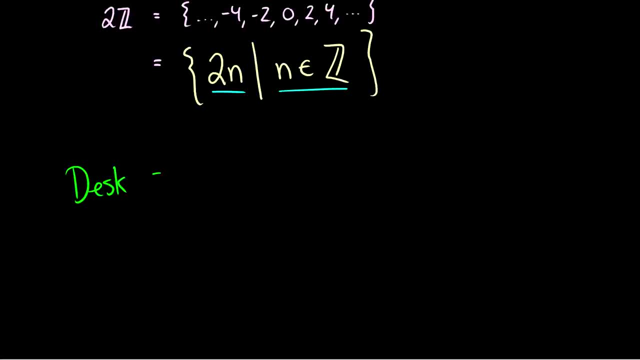 I have a desk And on this desk I have a drink, I have a laptop and I have a microphone And there's some other things on my desk that I could list, but let's just say my desk only has these three things. 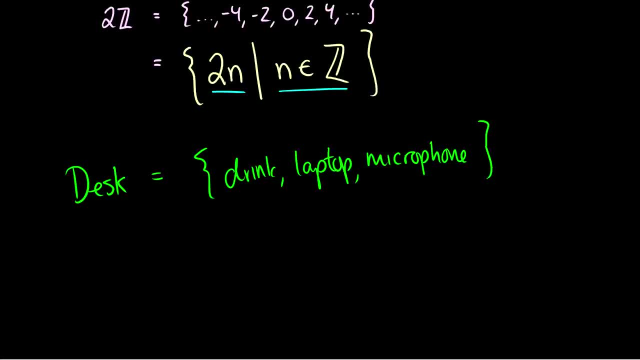 Now this is one way I can talk about things. I can say I got this drink, this laptop and this microphone on my desk. Or I could write this in set builder notation- if I might have a lot more things, or maybe I want to be vague. 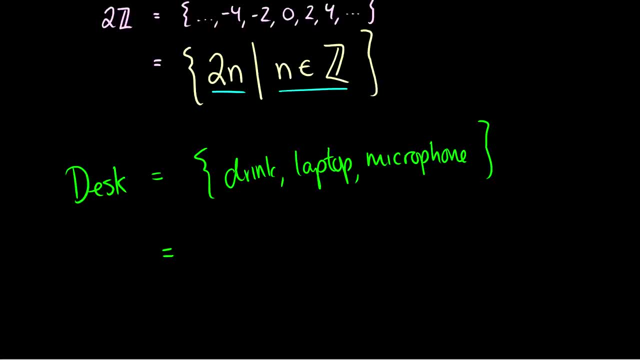 or maybe I'm not entirely sure what's on my desk, but I know there's things on my desk So I could rewrite this as the set of x. So this is a variable x, And what's the condition for x? x is on my desk. 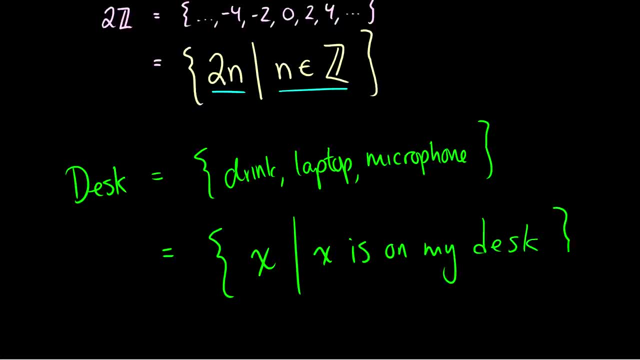 Yeah, so this is kind of cheating, right, But they're the same sets. So the first one, I'm listing all these items individually. The second one I'm saying: look, it's the set of variables x and whatever x is. 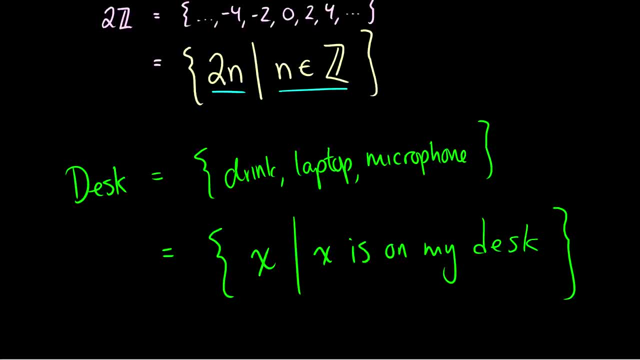 it just happens to be on my desk. So everything that's on my desk, it's just going to shove it in as x and it's going to build a set with it. So that's the set, builder, notation And, of course, mathematically, 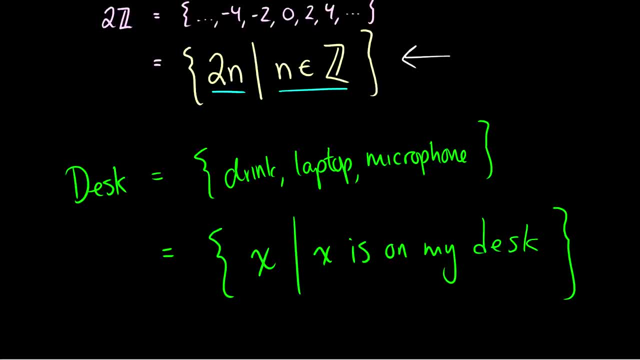 we do this very formally with, of course, numbers and formulas and notation, While, of course, if you do a linguistics example with words, it's much more wordy, it's much more flexible, much more floaty, But they both convey the same meaning. 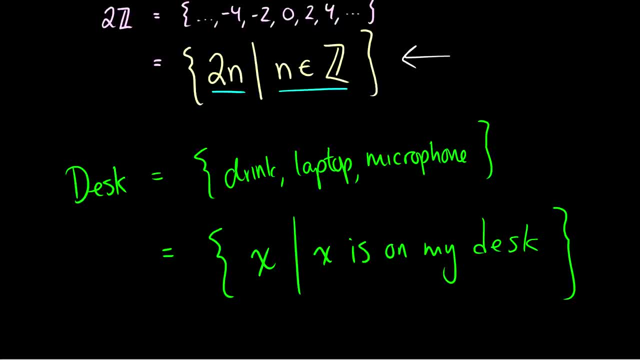 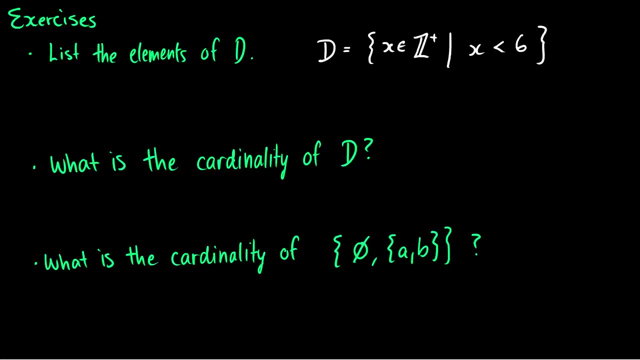 So if you didn't quite understand the mathematic example, then hopefully you'll be able to translate this desk example back into the mathematics after, while maybe understanding this at a more fundamental level. So here I have some exercises, And these all refer to the 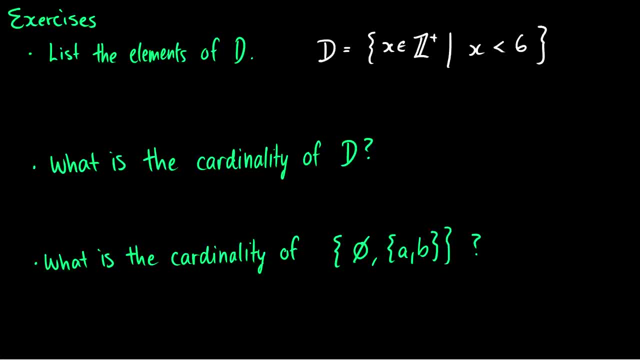 or the first two refer to the set D, and the third one is completely different. Try them yourself and if not, well, I'll give you the answers now. So list the elements of D. D is the set of x in positive integers. 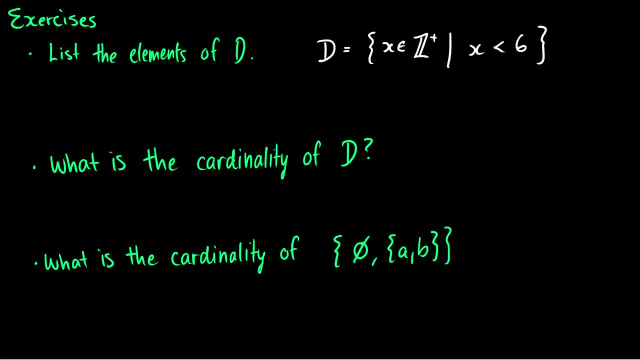 such that x is less than 6.. So I'm going to take all x less than 6 and add them to the set if it's a positive integer. So this means that I can have 1, because 1 is a positive integer. 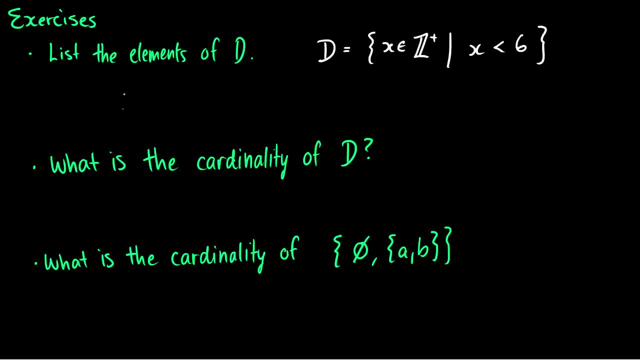 and it's less than 6.. Let's do this in a different color: 2,, 3,, 4, and 5.. Can I add 6?? I can't add 6 because x is not less than 6.. 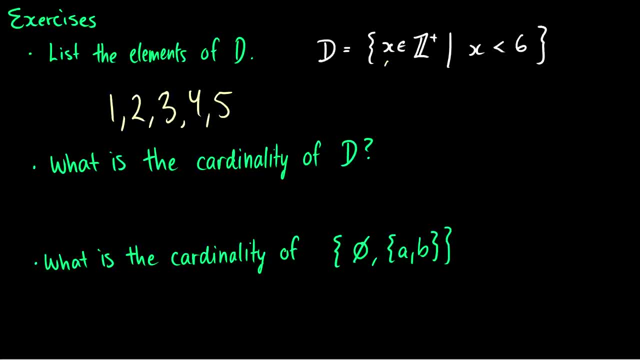 Can I add 0?? Well, I can't add 0, because I specifically want the x's that are in positive integers, and 0 is not a positive integer. Okay, what's the cardinality of D then? Well, this is easier. 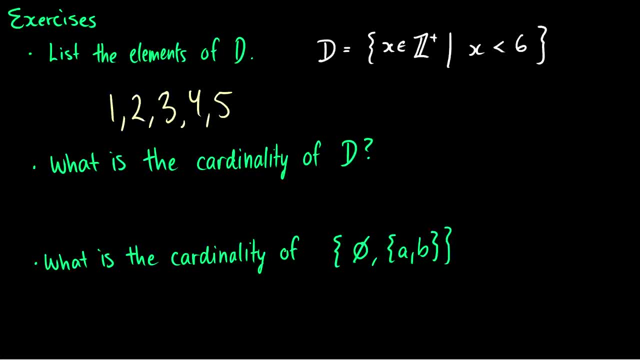 because I've already written out all the elements in my set. So I see there's five things there. So I can say the cardinality of D is equal to 5 because it contains the numbers 1,, 2,, 3,, 4, and 5.. 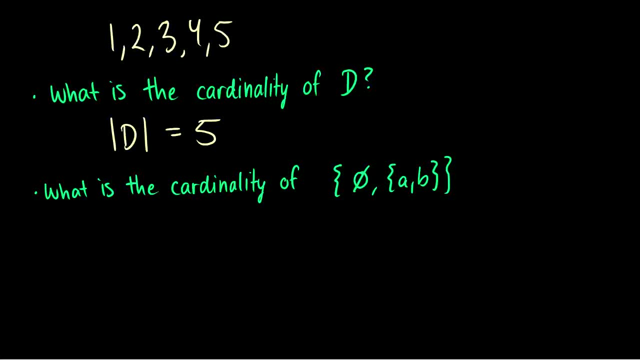 Now here's another question, and this is what I alluded to before: What is the cardinality of the set containing the empty set and the set AB? Okay, So how many elements are in the set? And when we look at sets, 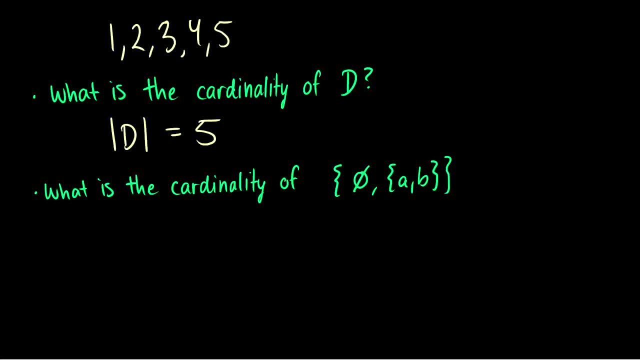 it's kind of like looking into a box and saying, well, what can I see? I see an empty set and I see another set. So really, what I see inside this box, if I were to draw this out, is a box containing nothing. 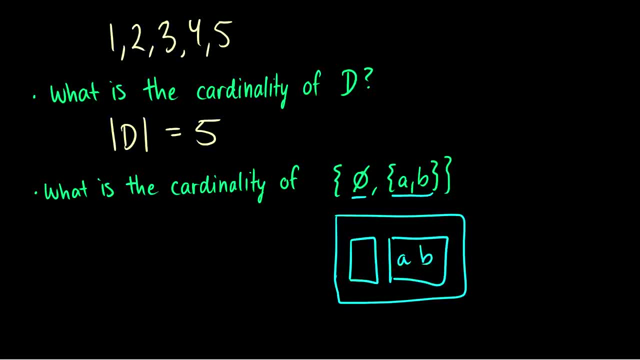 and a box containing A and B, So the stuff inside of these boxes, essentially with a cardinality question. these things are invisible, We can't see what's going on. So the question is, how many things do we see inside that set? 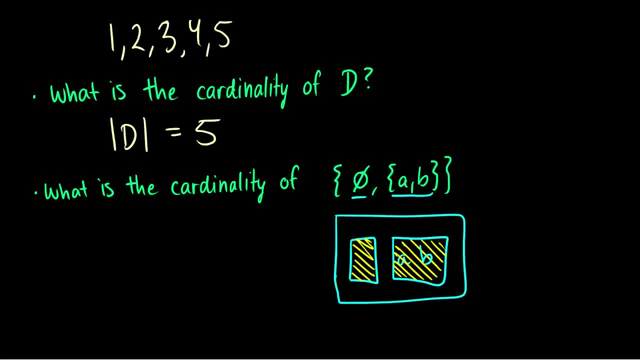 What is the size? How many elements are in that set, that big box? And the answer to this is two, And this is why I said: look at the commas here. So we have an empty set, which is the first thing.